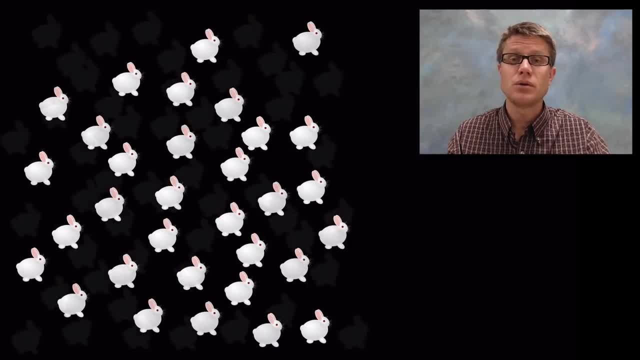 rate of 1.. And so we're going to now have 16. And now we're going to have 32.. And now we're going to have 64. And we're going to have 128. And we're going to have 256. And 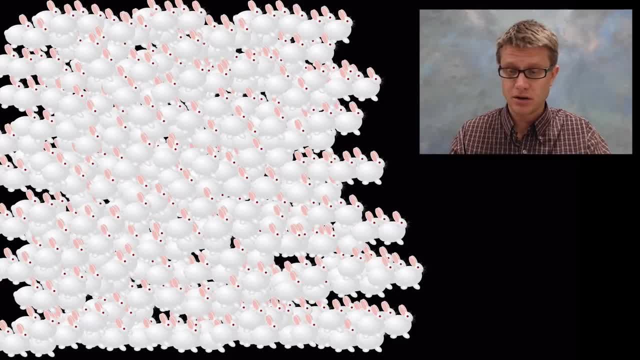 pretty soon my whole screen is going to be filled with rabbits, And I heard my fan come on on my computer because it's really taxing to put that many rabbits on the screen. And so does that occur in nature? No, And Darwin noted that as well. He looked at instead. 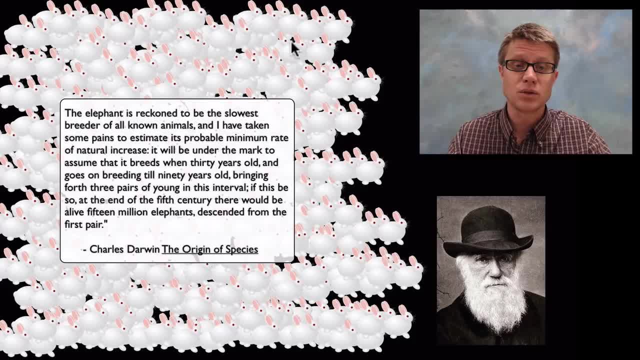 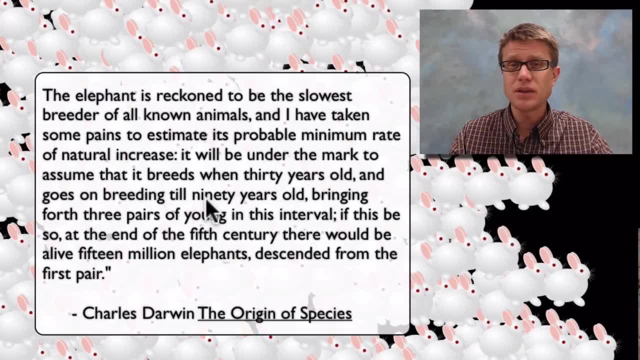 of rabbits, elephants. Elephants take a long time to reproduce. In other words, they have to be 30 before they can reproduce And they live until they're about 90. And what he found is that, even though they might produce three pair of offspring during that period of time, if you just let them keep. 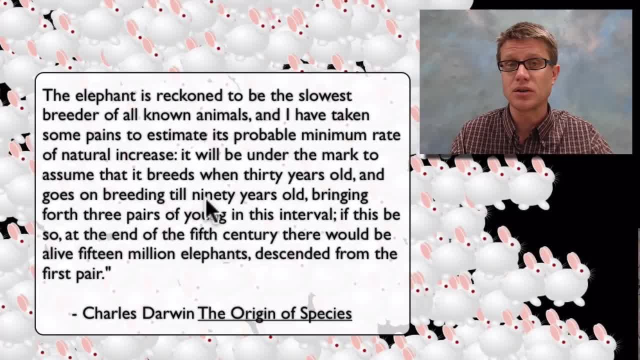 breeding over and, over and over again. after five centuries, or 500 years later, you're going to have 15 million elephants, And so exponential growth goes really, really quickly, And we know that it can't last forever. Eventually we're going to hit a limit, And so let's look. 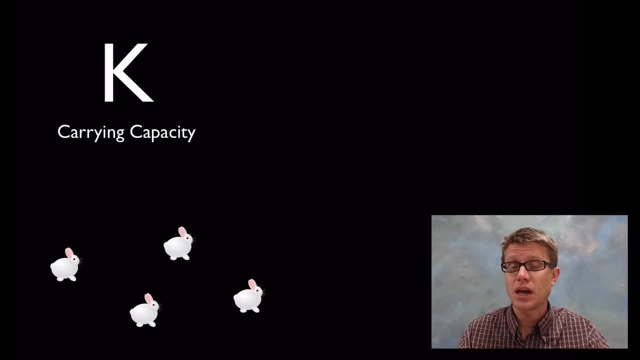 at those four rabbits again. Eventually they're going to reach what's called k or carrying capacity. It's the maximum amount of time that they're going to live And they're going to come out in a population that it can be supported in a general kind of in an ecosystem. 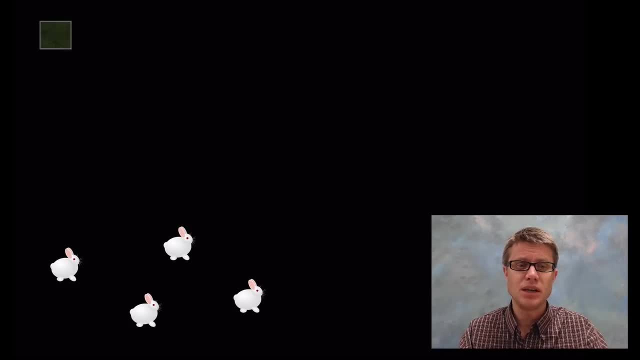 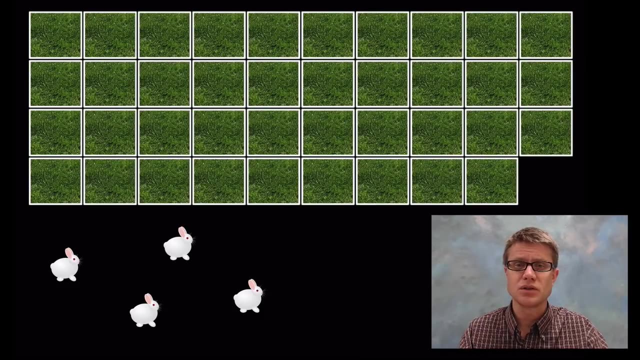 or in an area. And so why is that? Well, rabbits eat things, And that is grass, And when they run out of grass, they die. Now I don't have the ratio right. You have to have way more producers than you're going to have consumers, And so let's put our rabbits on the grass. 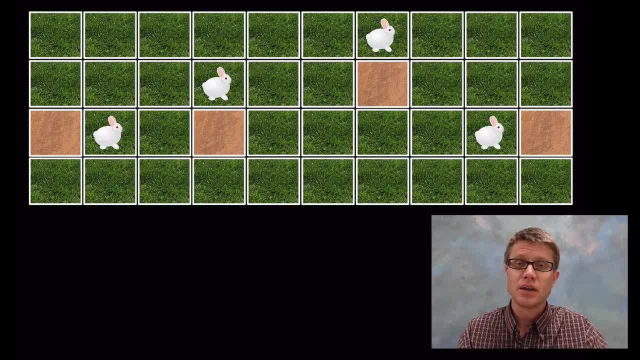 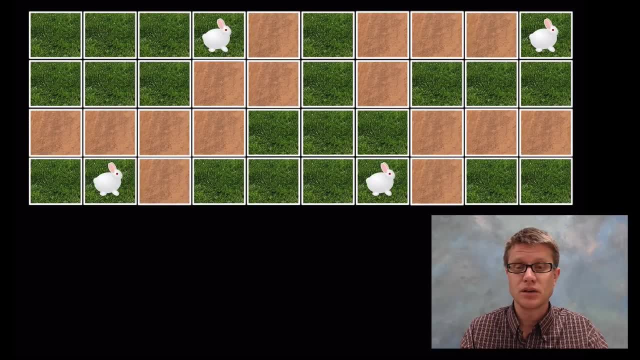 What are they going to do? They're going to eat the grass, And as they do so, that grass is going to go away and they're going to have to move on to another area, And so, luckily, there's more grass for them to find. But eventually they'll eat their way into the grass And 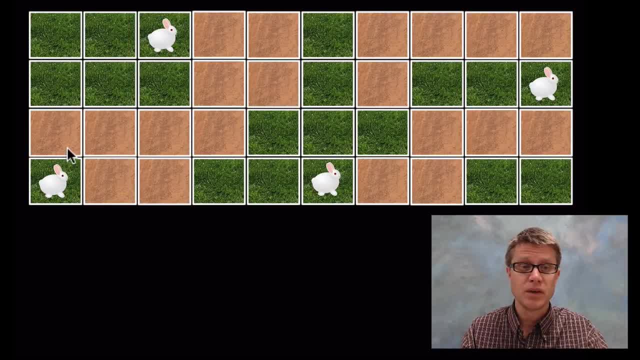 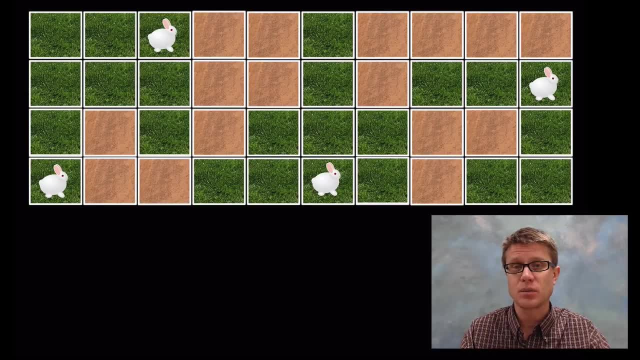 to a corner, And so this rabbit right here has a problem. If this grass didn't grow back, it would really be stuck, And so if we had much more than four rabbits, we would have exceeded the carrying capacity, And in class, I asked my students to build models that showed 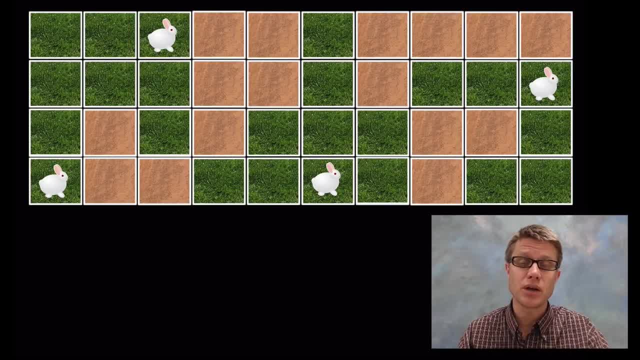 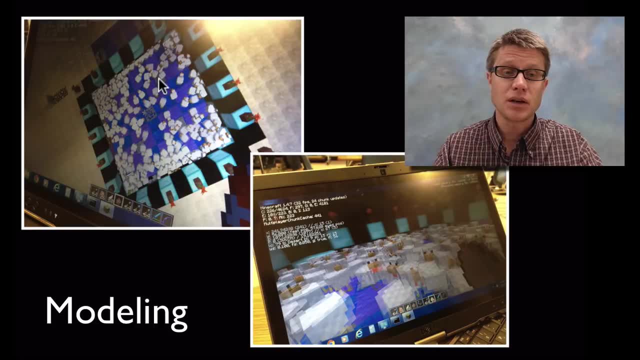 logistic growth, And a lot of them used paper and pencil, But one creative group used Minecraft And what they did is they constructed a little chamber here and they put one chicken in it, And every time the chicken would step on one of these platforms, two doors would open up. 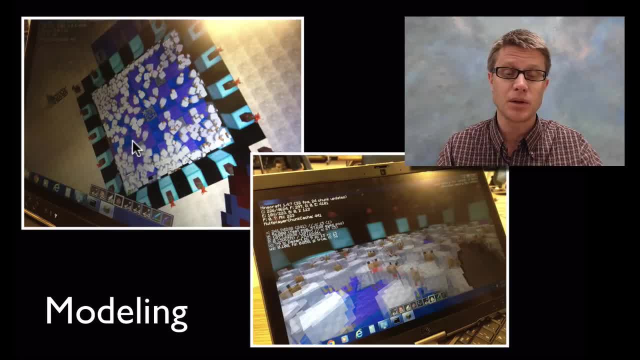 and two more chickens would come out. So pretty soon we had three chickens And they'd step on platforms and pretty soon we had five chickens And it just went really, really, really quickly. Pretty soon there were chickens everywhere And I asked them. well, it's got to show logistic growth And 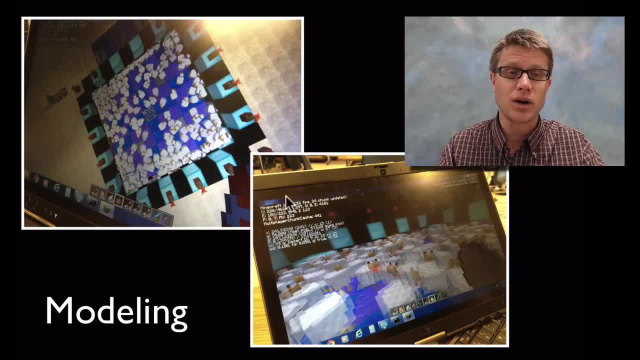 these bright students, Gabe, Ethan and David, said: well, watch what happens. Eventually, as they stand on the platforms, it becomes so crowded they can't get off anymore, And so they can't release any more chickens into the area. And so eventually it reaches kind. 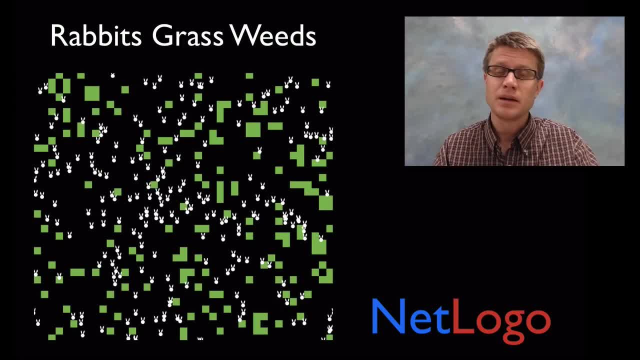 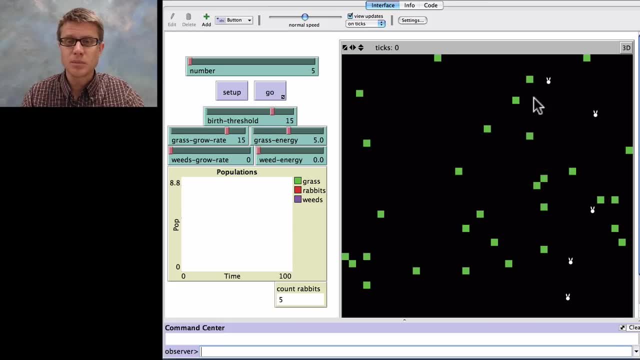 of a carrying capacity of chickens in this one container. Now let me show you another model. This is a NetLogo model called rabbits, grass and weeds, So let me launch that for a second. So in this model, the rabbits are going to be these little white things with 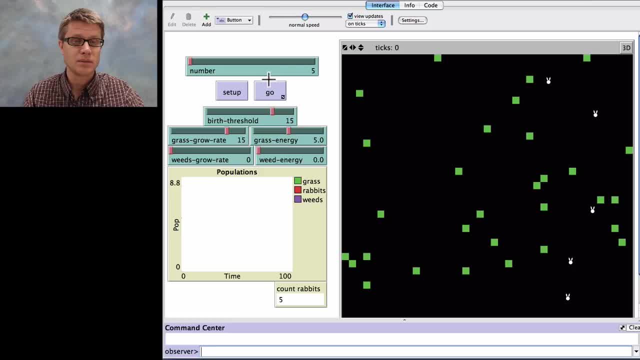 ears, And then the grass are going to be these little green squares, And so we start with five. Now the rabbits are going to find grass if they can, And if they can they're going to get energy, And if they get enough energy they can breed. But if they don't find enough, 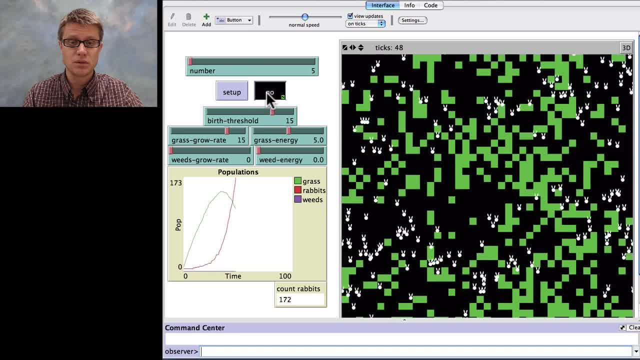 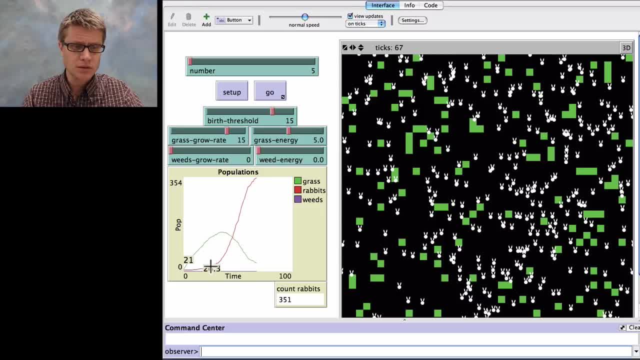 going to represent the number of rabbits over time, And so, again, we started with five, And pretty soon we had 350 rabbits. What happened to the grass? Well, the grass started to reproduce as well, but it crashed because the rabbits were eating all the grass. And so let's watch. 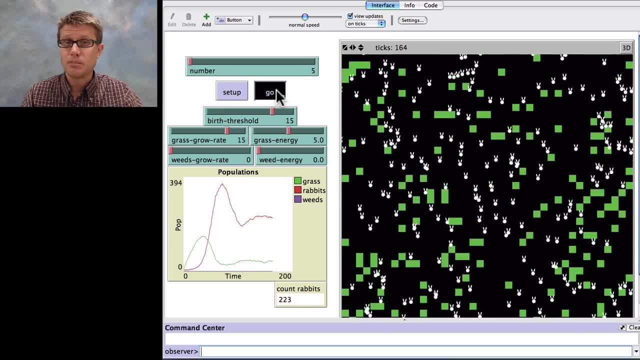 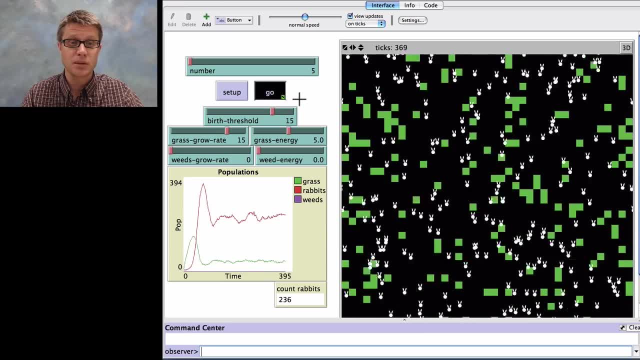 what happens now if we let it roll for a second. So we're going to see a big drop in the number of rabbits And then it's going to finally hit a limit. So we're going to find like a perfect amount of rabbits that we have. So we're reaching what's called carrying capacity. 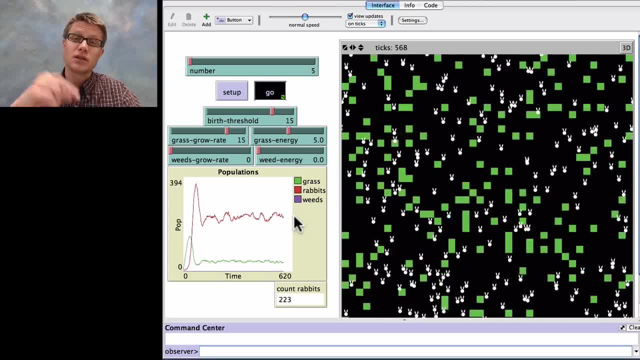 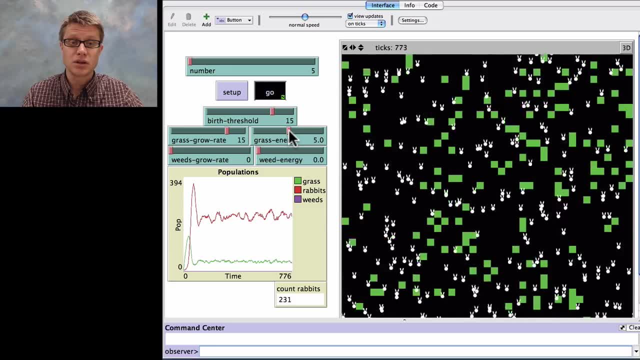 And you can see that if we let it go over and over and over the grass and the rabbits are going to go up and down, But we're going to reach a limit. Now let's say that we gave the grass more energy. So if there's more energy in the grass, let's increase that. 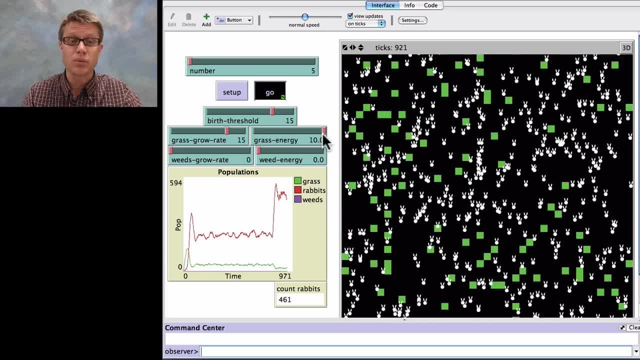 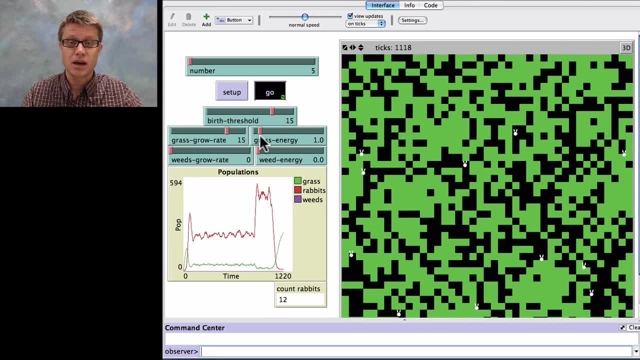 we're going to see exponential growth again And then we're going to have even more rabbits. Or let's say we said that the grass has less energy. As we decrease that, then we're going to have way fewer rabbits And so that rabbit population is going to drop, but it's going. to find another carrying capacity. And so what happens? You're going to see something here. It's a little more dense, Just a little more dense, And it's going to start to go up and down again. And if you look at that, you'll see the grass is going to go up and 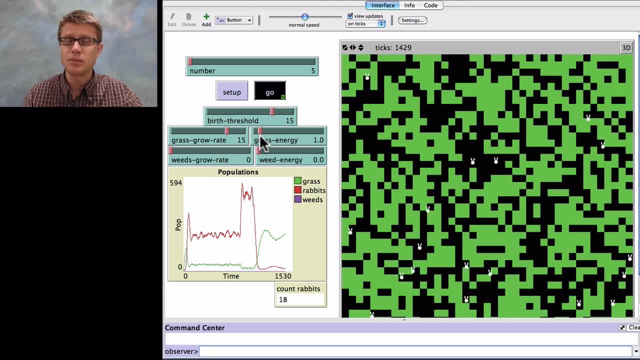 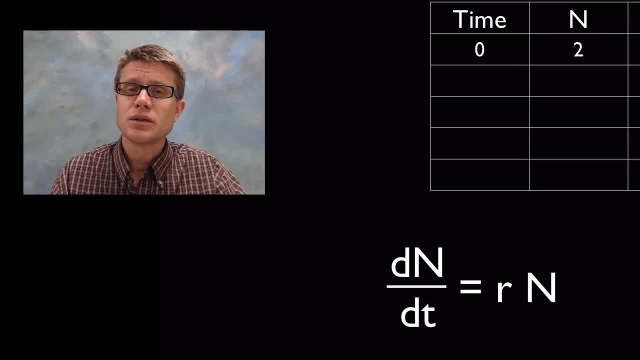 happens, as your population size increases, you run up against these limiting factors, And those limiting factors are going to slow your growth. So let me quit that. So let's get to the math now. So if we're looking at exponential growth, so exponential growth. 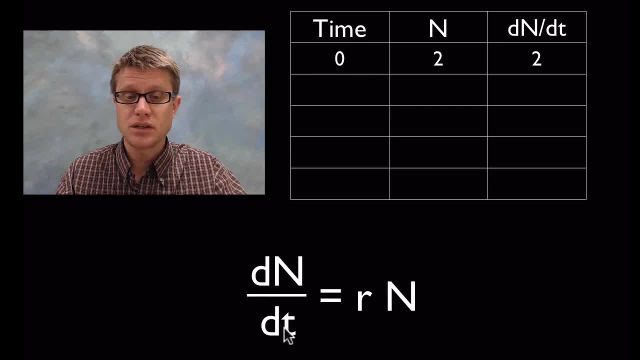 the equation is going to be this, right here, And so dN over dt means the change in N over the change in time, And so it's going to be R times N, where R is the growth rate and N is the population size. And so if we started, like we did at the beginning, with exponential, 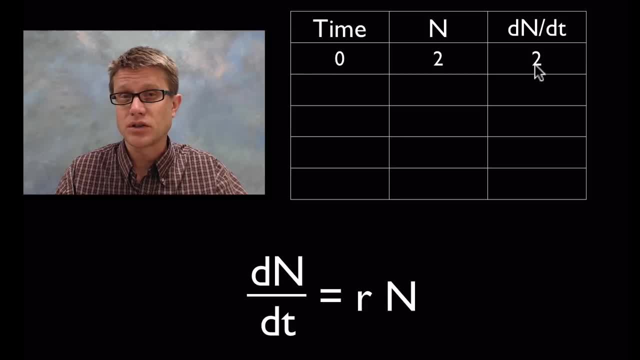 growth. you're going to have two rabbits. What's our change in N over change in t? It's going to be 2.. How did we get that? We're multiplying R, which is 1, remember, times N, which is 2.. And I'm going to get 2.. What happens to that change in N? Well, that's going. 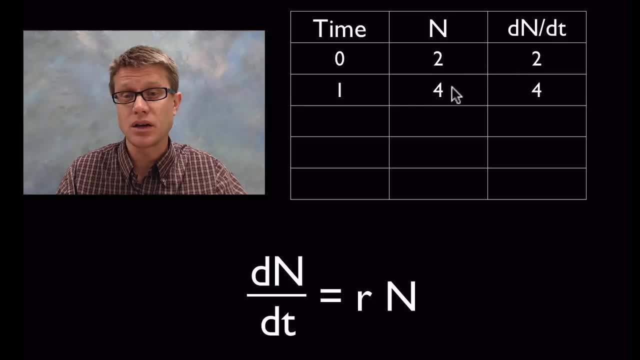 to give me my new population. So I'm taking 2 here plus 2 here, And now I have 4.. What's my change in N over time? for the next one, Again, since our R is 1, it's going to be: 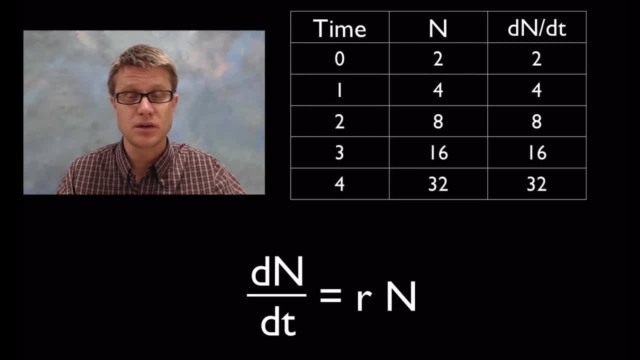 4 again, And so we're going to have 8.. We're going to have 16.. We're going to have 32.. So if we were to graph that, that's going to give us that J shaped curve. But what I? 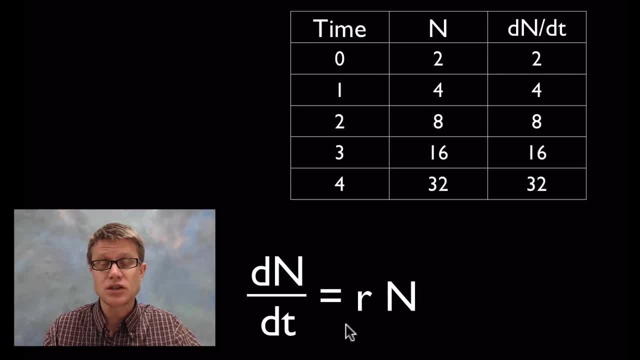 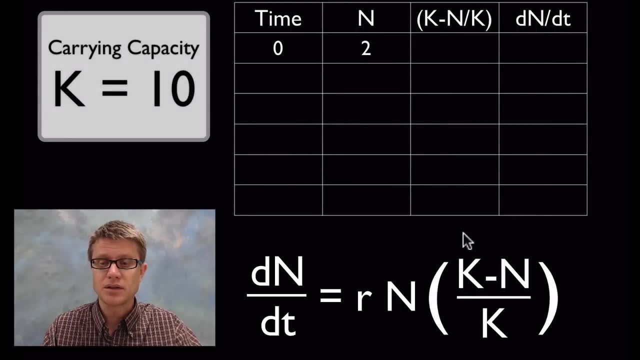 want you to do is look at this equation right here and watch as I change it to an equation that shows carrying capacity, And so the only thing that's going to change is what's in the parentheses right here, And so that's going to be the factor that's related to carrying. 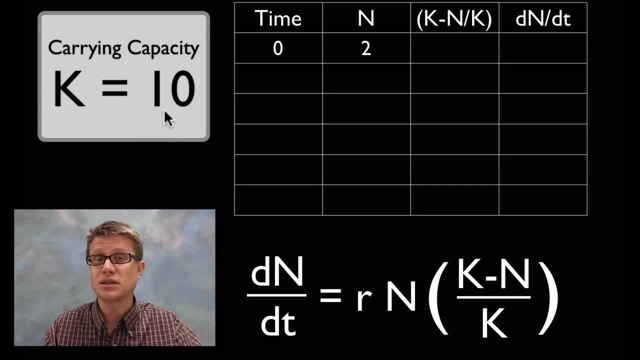 capacity. And so I'm going to choose an arbitrary carrying capacity. Let's say it's 10.. That the area can only support 10 rabbits. Let's watch what happens. And so we start with 2 rabbits, And so I'm going to show you what's in the parentheses. 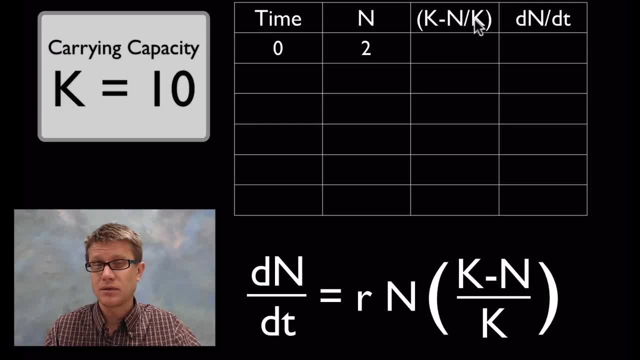 here. And so we're going to have k minus N divided by k. Well, what's k? What's our carrying capacity? That's 10. Minus N. So that's minus 2. So we're going to have 8.. And then what's? 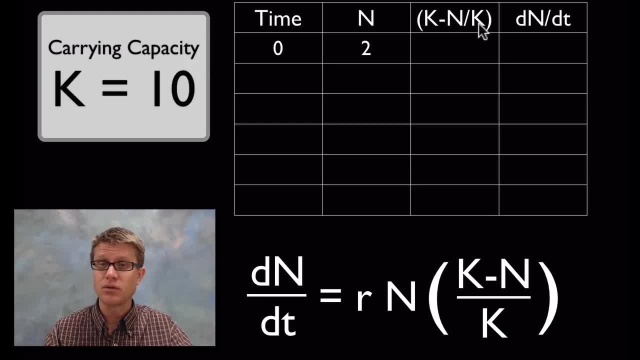 our carrying capacity. It's 10.. So it's going to be 8 divided by 10.. Or it's going to be 0.8.. Okay, Now we're going to figure out this. And so what's this? It's R, which we said. 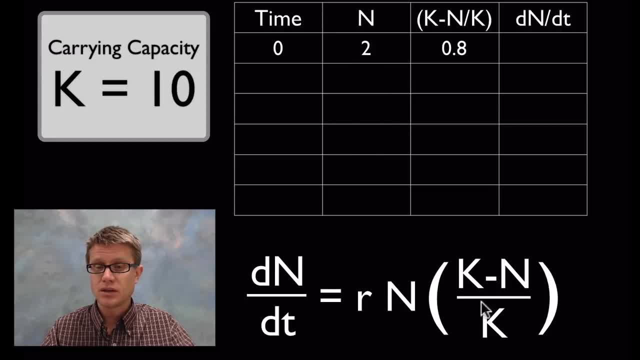 was 1, times N, which we said was 2., And so we're going to have 8 divided by 10.. And so it's going to be 2 times what's in this parentheses, which is 0.8.. And so that's going to be 1.6.. 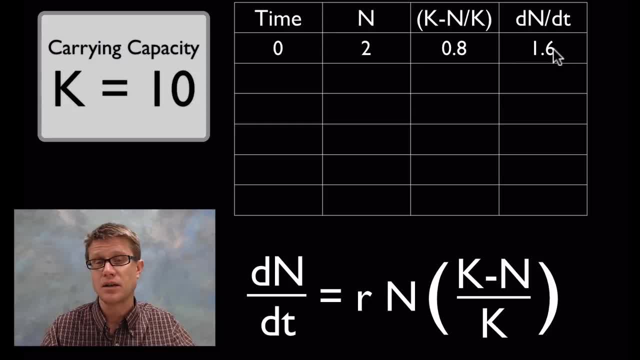 And so this whole equation tells us how many new rabbits we're going to add, And I'm not going to round so I can show you what happens as we increase this, But know this: that we're going to increase it by 1.6 rabbits. So let's look at time 1. Now we have 3.6 rabbits, Where 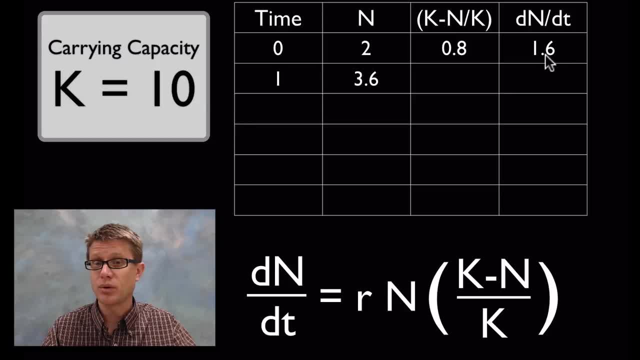 did I get that? It's the two original rabbits we had, plus the 1.6.. Okay, What's going to be in the parentheses now? It's going to be k, which is 10, minus 3.6.. So that's going. 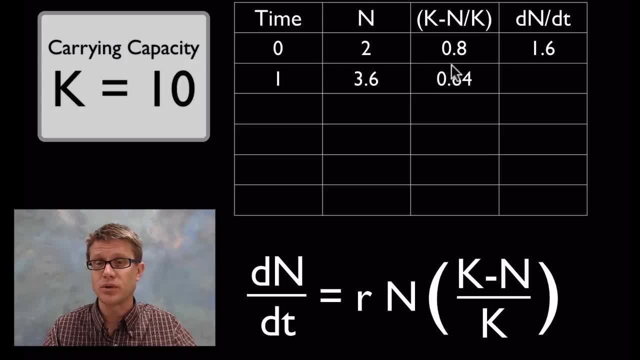 to be 0.6.. So that's 6.4 divided by 10.. Now it's 0.64.. You can see that that number became a smaller number. We're going to multiply that times 3.6.. Again, it's 1 times 3.6 times. 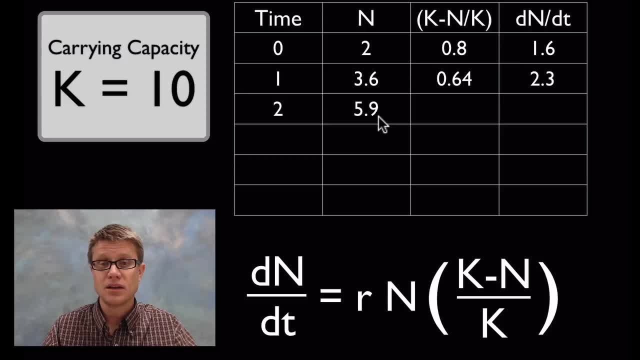 that value And we get 2.3.. I'm going to add that to our original 3.6, and now we get 5.9.. What's going to be our k minus N over k? It's going to be 0.41.. And so what do we get? 2.4.. 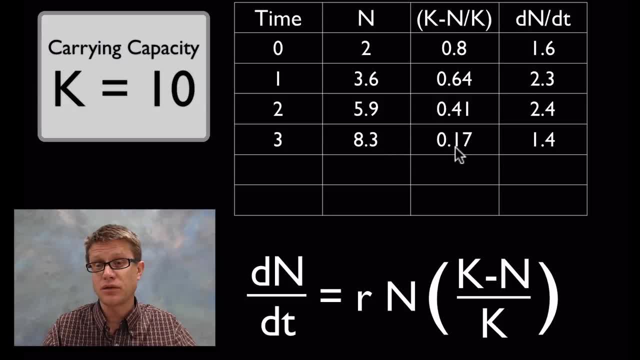 And so you can see that, as the population is increasing, this factor is becoming smaller and smaller. And so now we're only adding 1.4.. And now we're only adding 0.29.. And now we're only adding 0.009.. And so what's happening to N? You can see that it's increasing quickly, right? 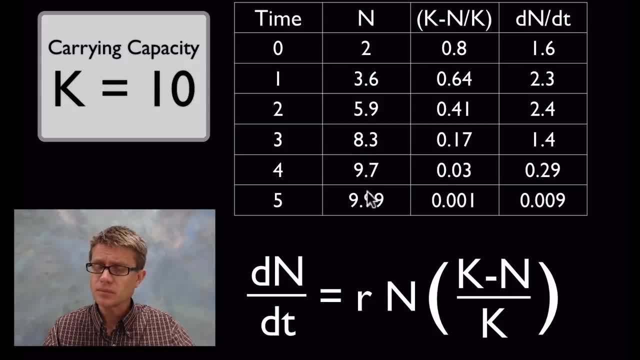 away, But the closer we get to that carrying capacity, it's kind of leveling off And it's reaching that limit at that one point. So this is just mathematical, It's not a model, But it shows that we're eventually going to approach that point. And so again in review: 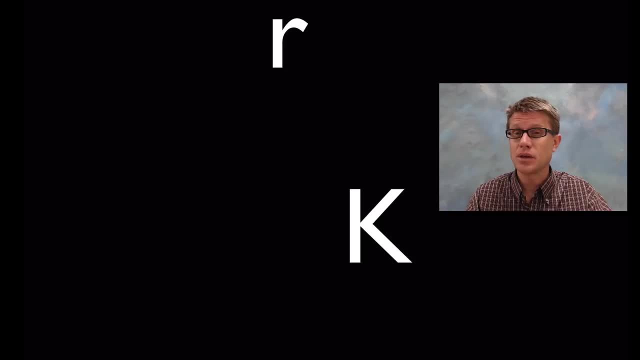 what's r? r is going to be the growth rate. What's k? k is going to be the growth rate, k is going to be the carrying capacity. So if our r is ever greater than 0, remember, we're going to show exponential growth. And if we ever have k, if we ever have a carrying 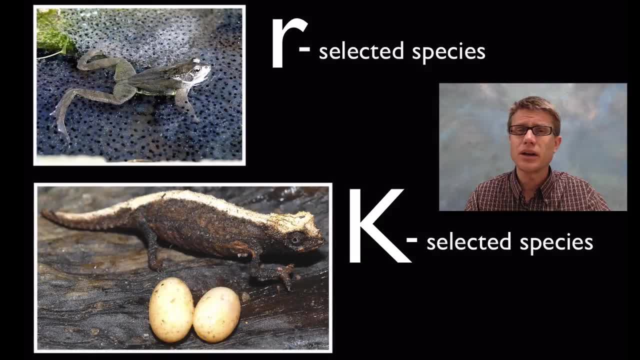 capacity. we're going to show logistic growth, But we also have species that specialize in these two. We've got r selected species and k selected species. So what does that mean? An r selected species is going to be a species that loves to grow as quickly as it can Look. 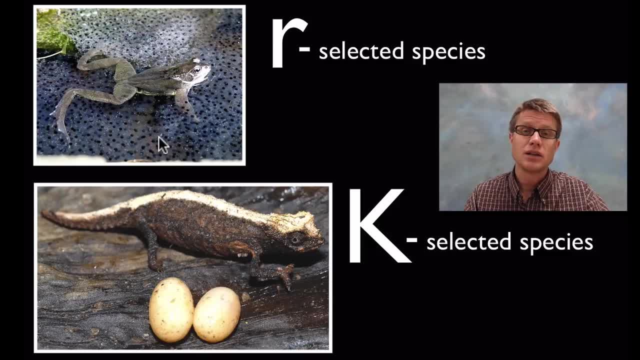 how many babies this frog is going to have. Thousands of those, And then we have the other, And so if I were to take this frog and introduce it into a pond where there are no frogs, we're going to have a bunch of frogs really, really quickly. We're going to have an r. that's really. 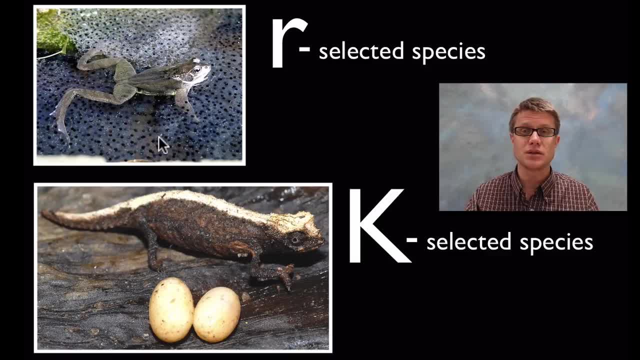 really large And they're going to fill that area. They're going to run out of resources and crash And they're going to boom and bust, But they're going to fill it really, really quickly. If we were to look at this, which is a chameleon? a chameleon is going to only 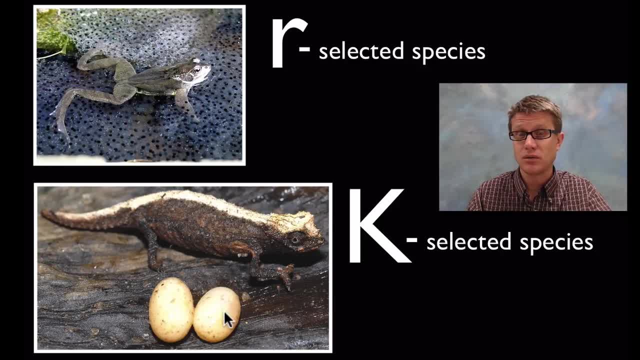 have two offspring, So its growth rate is going to be really, really slow. What is it going to do? It's going to give them a lot of parental care. It's going to invest a lot of energy in just its few offspring, And they're all going to survive. If we look up here, 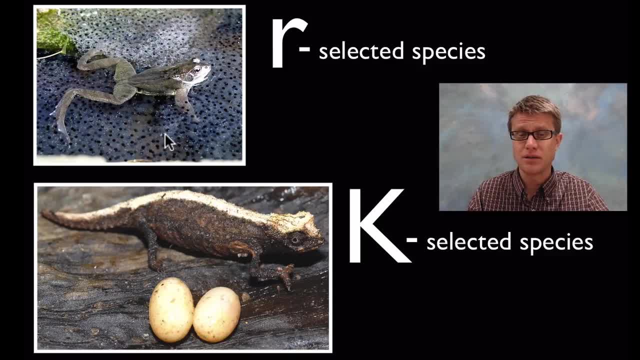 with r selected species. most of those are going to die eventually, But with this chameleon, since it's taking so much care of them, it's going to take very good care of it And they're all going to survive. This is going to gradually increase and find a nice carrying capacity. 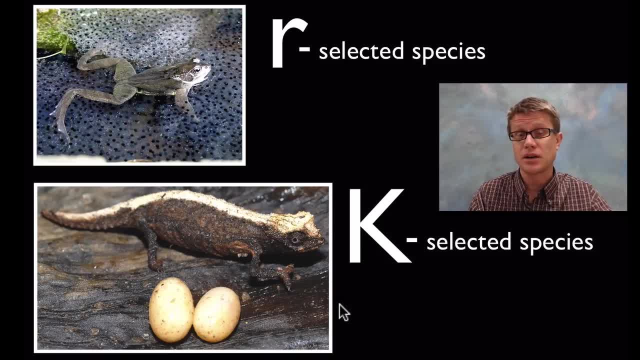 So what are we? What are humans? Well, we invest a lot in our young. A lot of my students are 17 years old and they still live at home and their parents take care of them, So we're really investing in them. And so what kind of a population curve are we going to see? 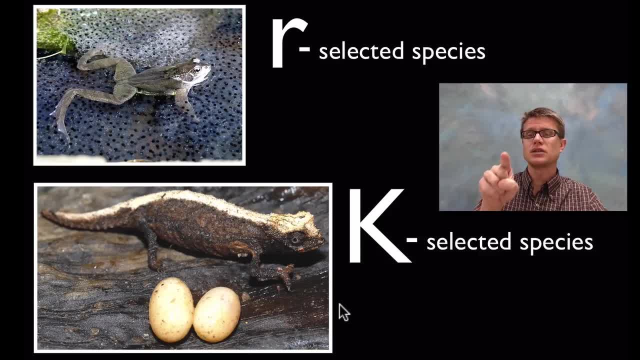 We're going to see an increase in the population. We'll see a lot more young people. We'll see a lot of older people. We'll see a lot more young people. We're going to see a lot more young. correlation curve are we going to see in humans? We're going to see a gradual, exponential increase. 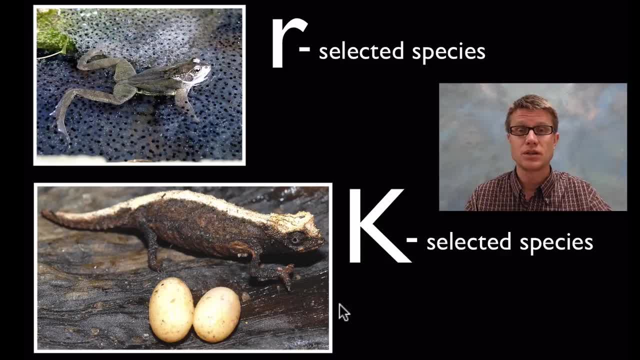 and then a nice carrying capacity which we're eventually going to reach, And we don't want to have this boom and bust cycle. So it's not so cut and dry as that. There are obviously species that are somewhere in the middle. So what about a tree? do you think A tree? 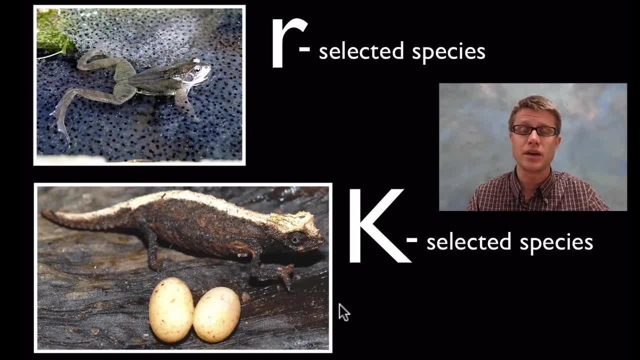 grows really slow, but they're going to produce a lot of offspring. And so what are they? There's probably no right answer for that. And so again, what is logistic growth? It's growing quickly, but eventually reaching a carrying capacity, And that's based on limits. in your environment And I hope that was helpful. 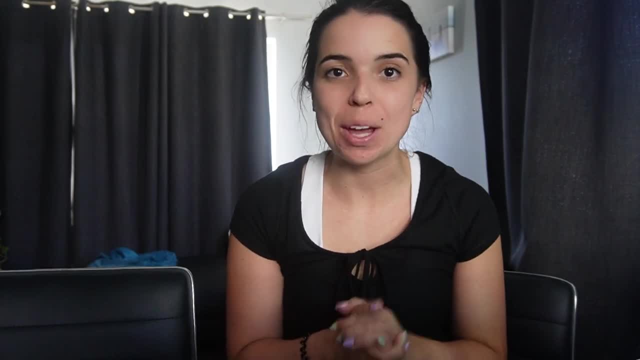 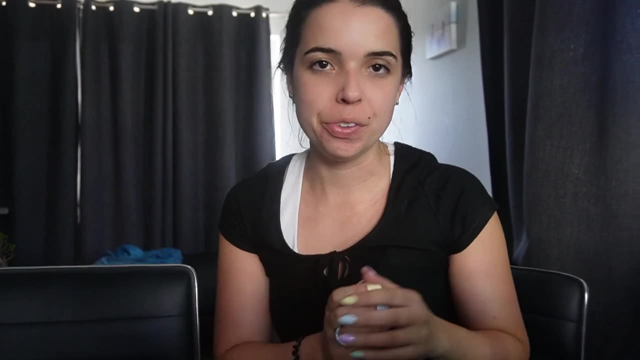 Hello, great tens, in this video I'll be introducing you to the topic waves, sound and light. This will be a very brief introduction video Videos to come within this playlist. I will go over the different types of waves, the theory behind those waves, formulas related to the calculations and we'll.